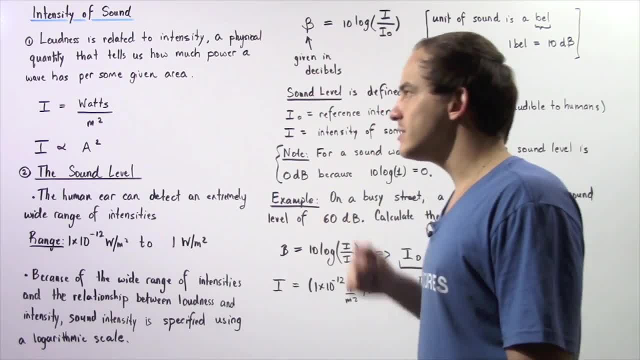 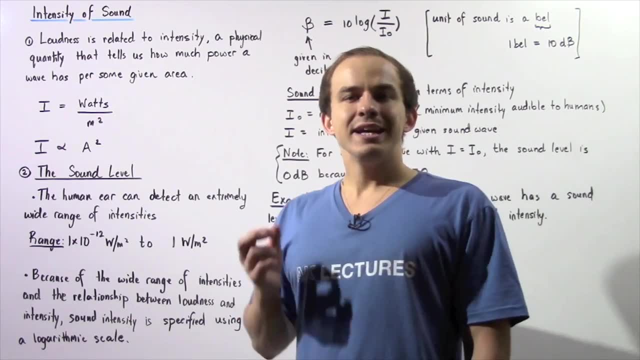 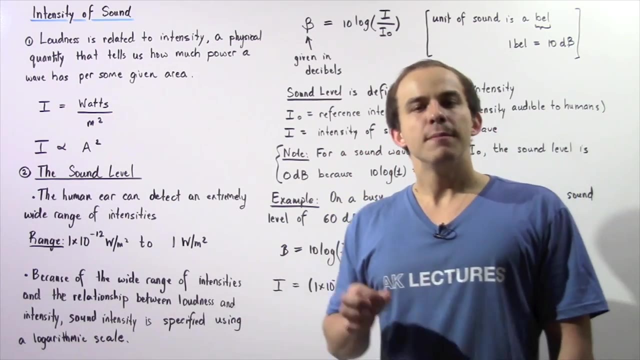 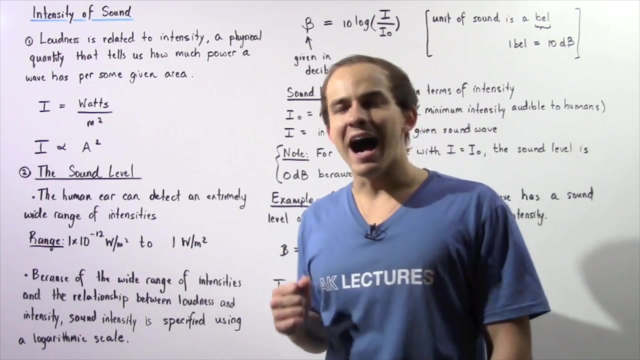 sound wave, we increase the loudness. If we decrease the intensity, we decrease the loudness of that sound wave. Now, the human ear is capable of detecting an extremely wide range of intensity values, beginning as low as 1 times 10 to the negative 12 watts per meter squared and going as 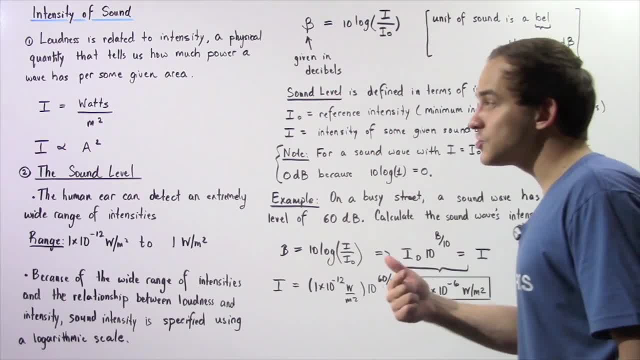 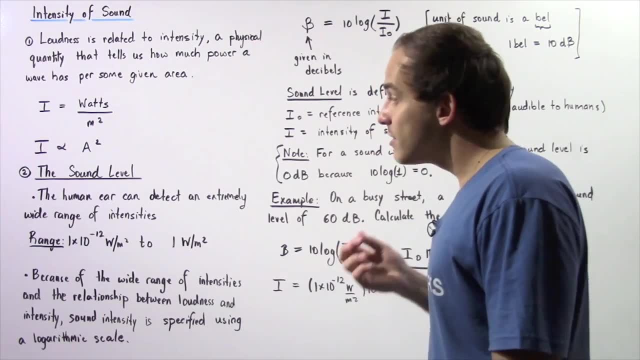 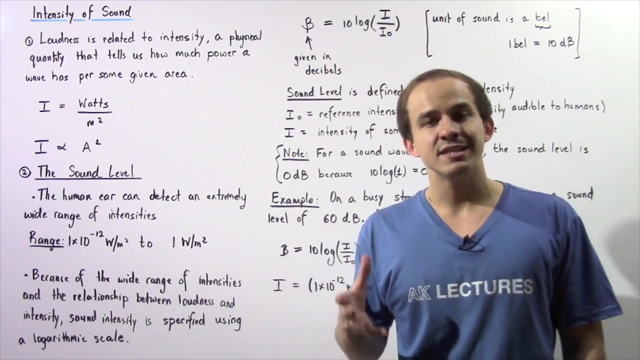 high as 1 watt per meter squared. Now, actually, the intensities can be even higher than this value, But if we go any higher, that will be extremely, extremely painful Now, because of this extremely wide range of intensities, of the human ear and 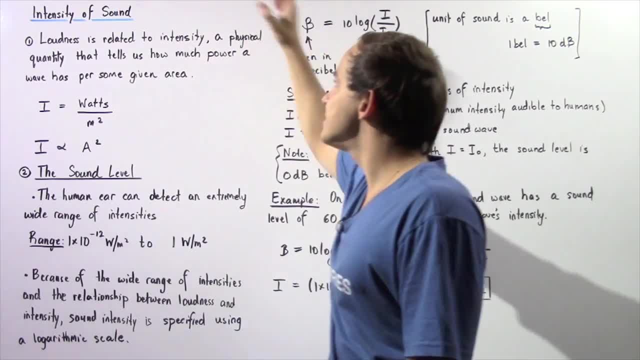 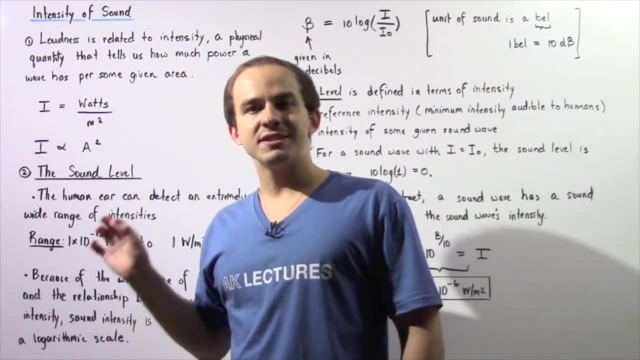 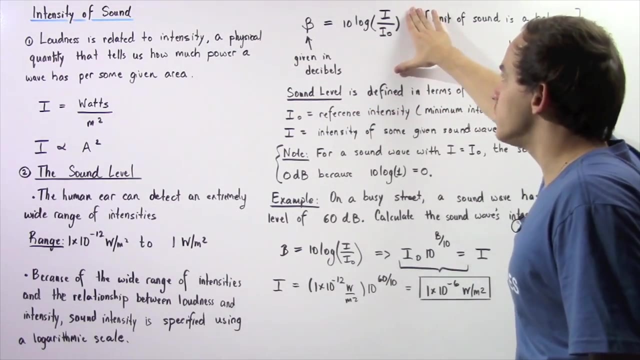 because of the relationship between loudness and intensity. we define our sound intensity using a logarithmic scale, And this is known as the sound level. So the sound level is given by the following equation: where the sound level is given by this capital: 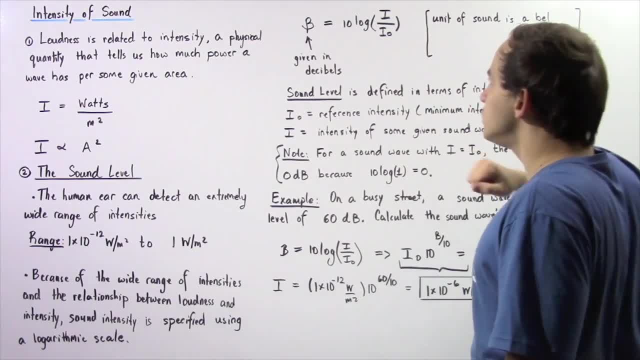 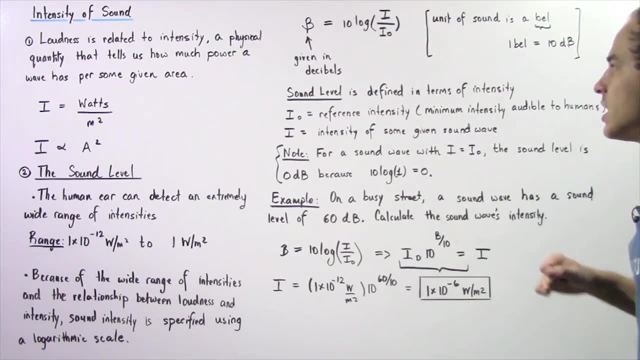 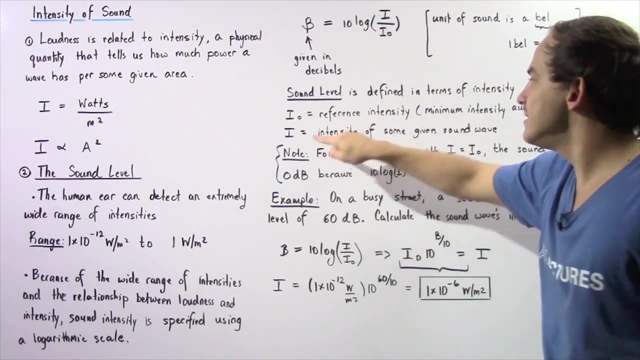 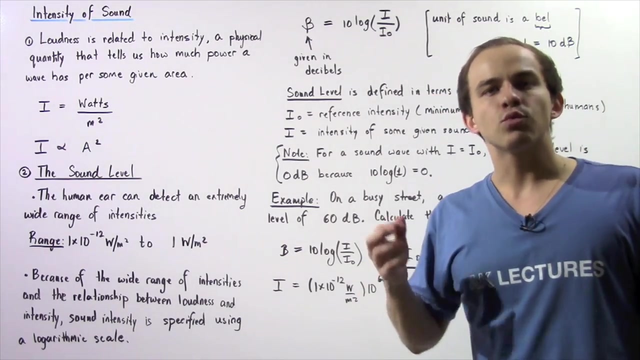 So the sound level is equal to 10 multiplied by the log of the ratio of the intensity I and intensity I0.. So the sound level is defined in terms of intensity of the sound wave. Now, I is simply the intensity of some sound wave that we're examining And I0 is simply a reference. 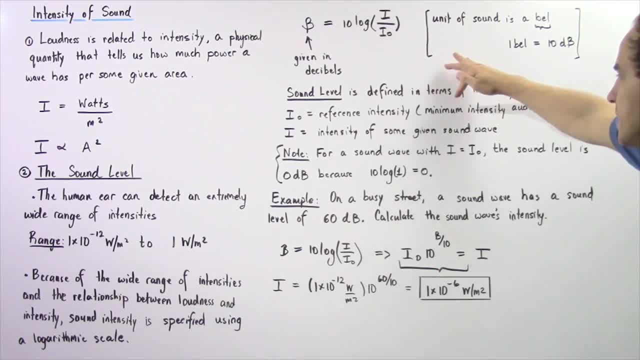 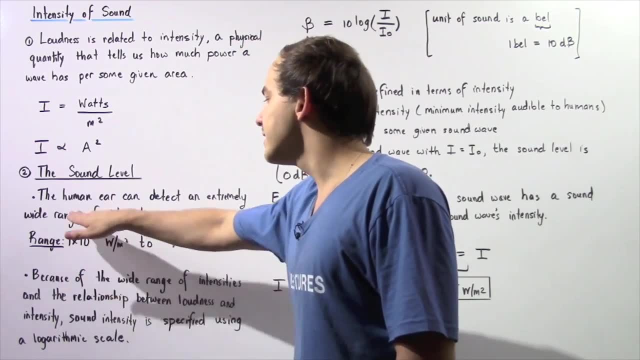 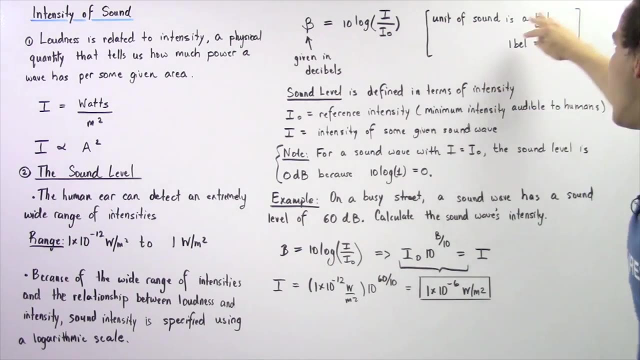 intensity. Usually, I0 is the minimum intensity of the sound wave And I0 is the minimum intensity audible to humans, And it's given by this quantity 1 times 10, to the negative 12 watts per meter squared. Now the unit of sound is given by a bell, And one bell is equal to 10 decibels, And this 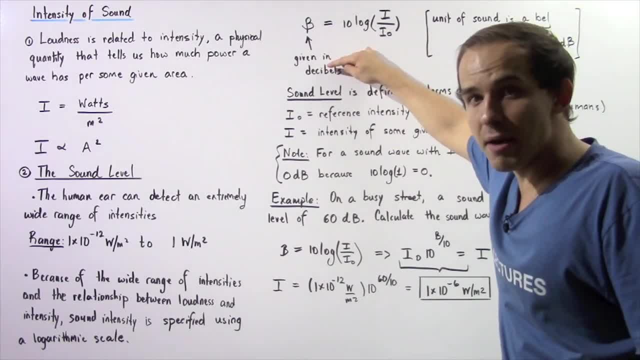 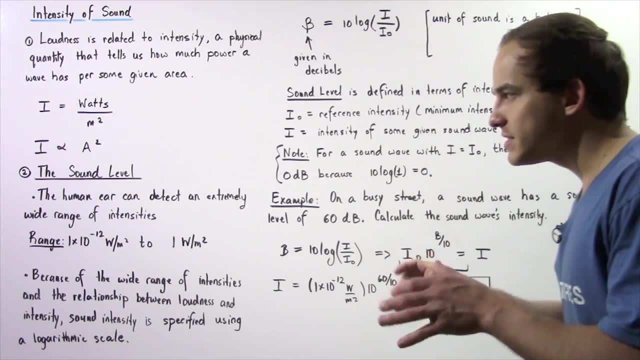 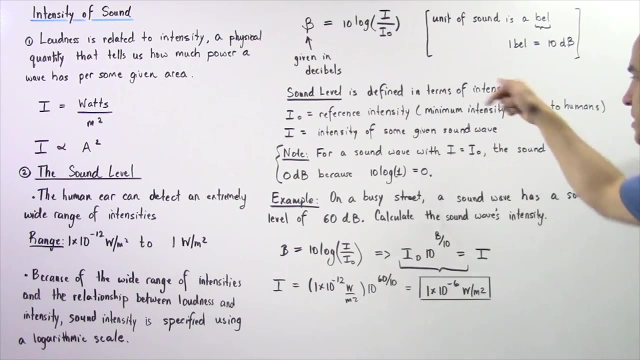 sound level B is given in decibels. So note the following: If we're examining a certain sound wave, that specific sound wave has an intensity that is equal to the reference intensity. in other words, if I is equal to I0, then the sound level is 0 decibels, And that's because 10 times log of 1 is 0. 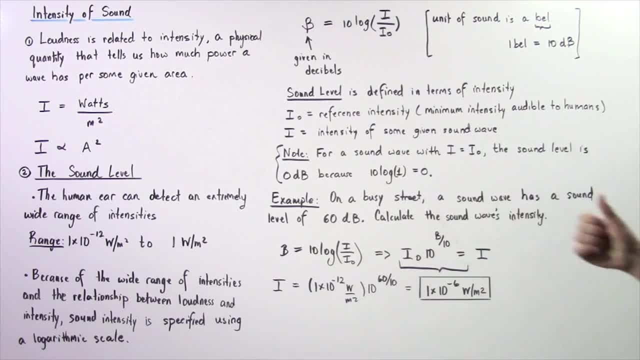 because log of 1 is 0. So let's examine the following example in which we're going to use this sound level equation. So on a busy street, a sound wave has a sound level of 60 decibels. Calculate the sound wave's intensity using the. 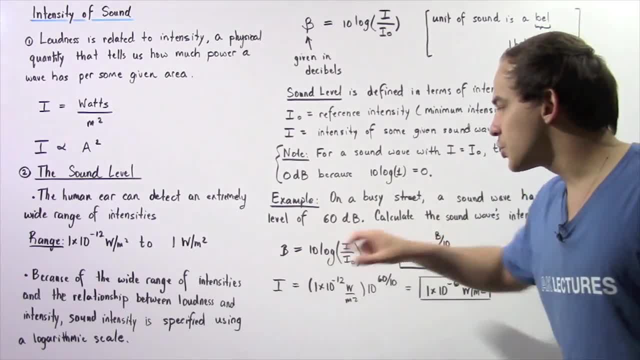 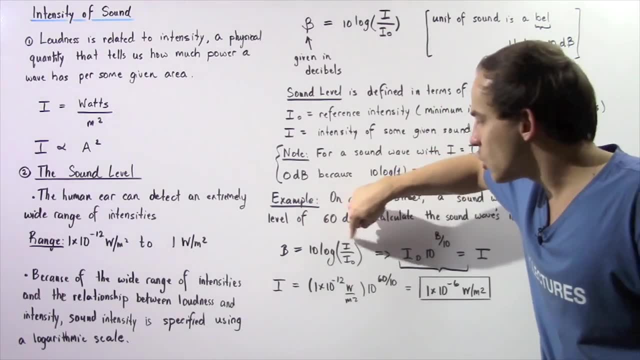 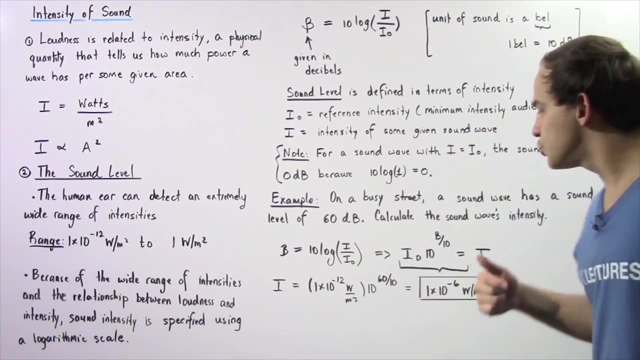 sound level equation. So we want to use this equation and we want to solve. we want to rearrange this equation and solve for I. So if we solve for I, we get the following result: I0 multiplied by 10 to the power of B divided by 10.. 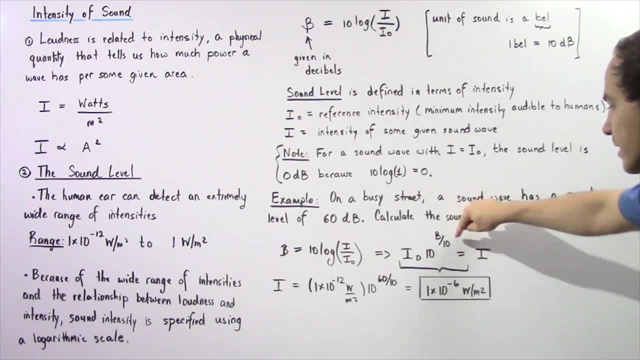 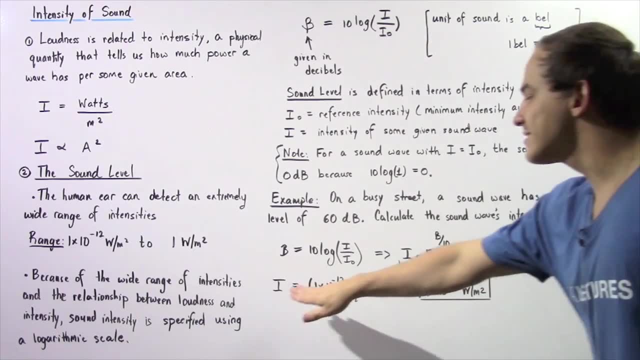 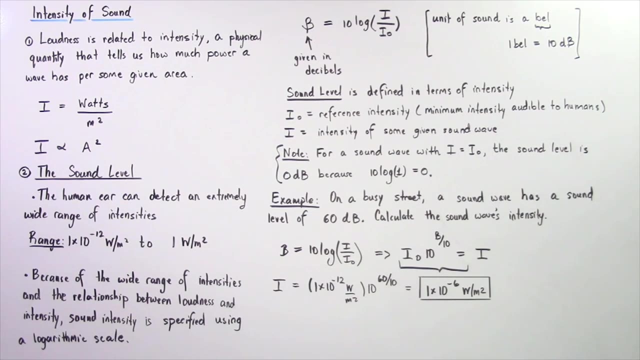 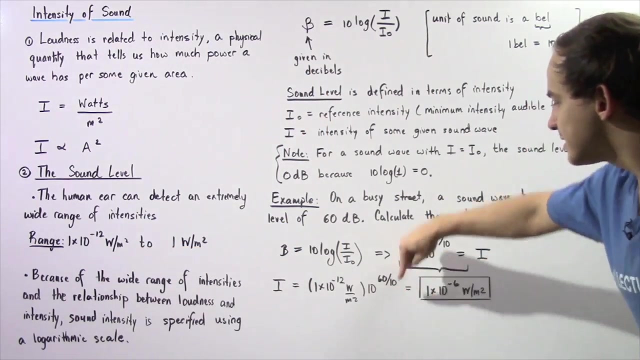 And where B is simply our sound level, this product is equal to I. So because we know what I0 is and because we know what our B is, we can solve for our intensity of that sound wave. Intensity is equal to the product of 1 times 10 to negative 12 watts per meter squared. this quantity multiplied by 10 to 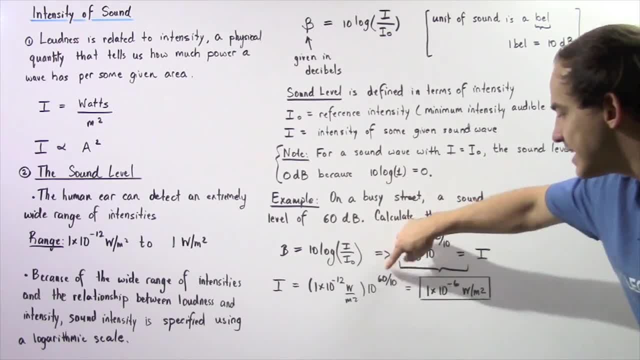 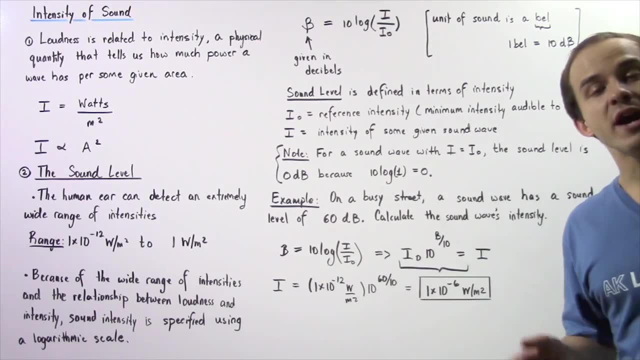 the 60 divided by 10. So 10 to the 6th power And we get a value of 1 times 10 to the negative. 6 watts per meter squared is the intensity of this sound wave. 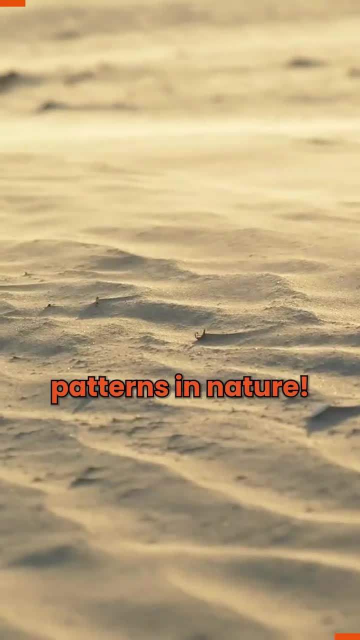 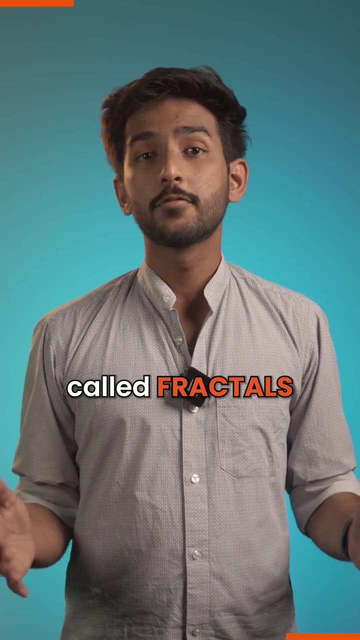 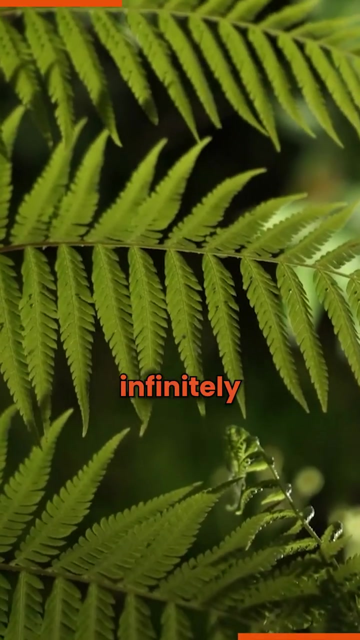 99% of people don't know about these mysterious patterns in nature. Have you ever observed the repeating patterns in seashells or snowflakes? These are called fractals and it can be found everywhere in nature. Fractals are patterns that repeat themselves infinitely, regardless of their size. 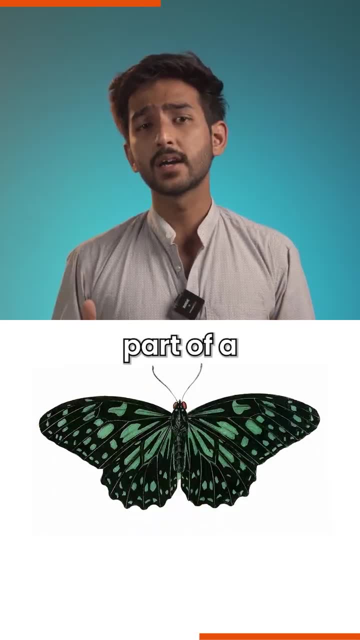 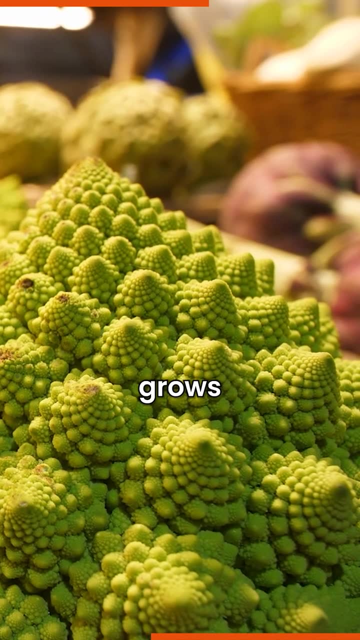 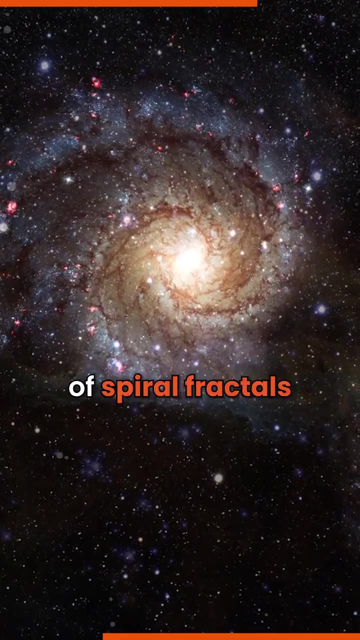 This means that even if you zoom in on a tiny part of a fractal pattern, it will look identical to the entire pattern. Your Manesco Broccoli, for example, grows in a spiral fractal pattern called the Fibonacci sequence. Galaxies are the largest known examples of spiral fractals.